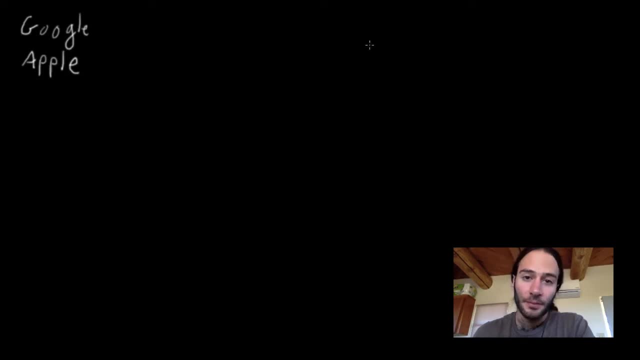 control of. Okay, so the first thing that's going to happen is we have Google. we'll put a little G here for Google And they could choose either to enter the market or not. So we'll put a little out here means they're not in the market And in and they are in. 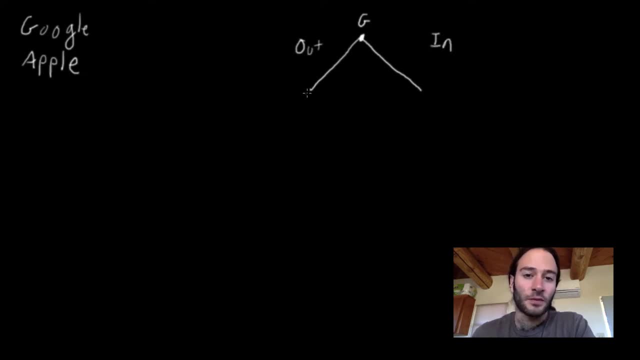 the market. Okay, let's see what happens if Google chooses not to enter the market. So after Google makes its choice, Apple needs to make a choice. we'll put a little A here for Apple. What Apple does is it chooses its pricing strategy. It can either be high or it could. 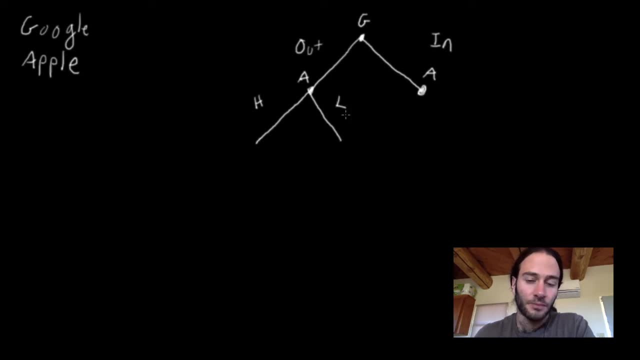 be low. Now, this is, of course, a simplification, But nonetheless it gets the point across. So now we want to say is: what are the payoffs When Google doesn't enter the market and Apple chooses a high price? Well, Google doesn't enter the market, they're not getting any. 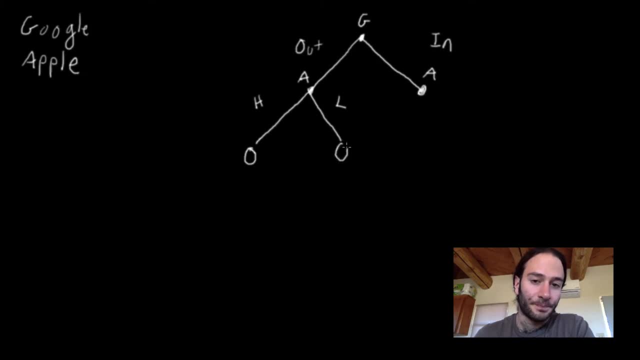 payoff. So in both cases Google gets zero. If Apple chooses a high price, well they get four because they have a monopoly, So they'll charge a higher price. If they charge a low price, they'll get, say, negative one. Okay, good, And just so we know Google is always the top payoff, Apple is. 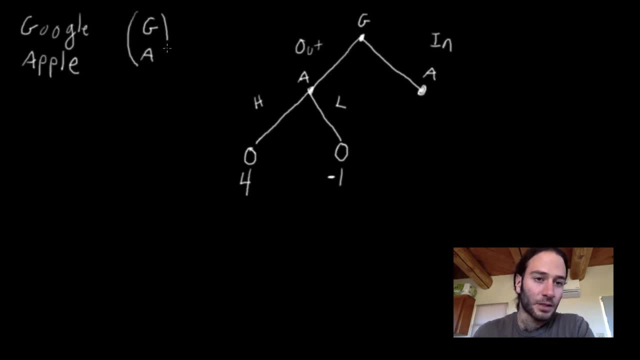 always the second one, So I'll do this. I'll put it in brackets or parentheses, and also put these in parentheses. you sometimes see this. Okay, so now, if Google chooses to enter the market, Apple still has to make the same decision. 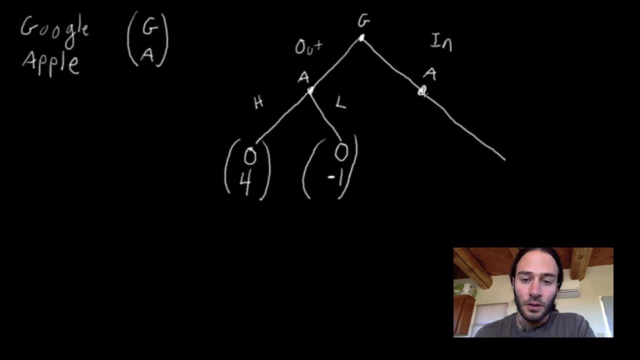 But now the payoffs are different. If Apple chooses a high price, it'll only get a payoff of two, because it'll split the market with Google, who is also getting a high price, who would also charge a high price. So the payoff to Apple and Google would both be two. 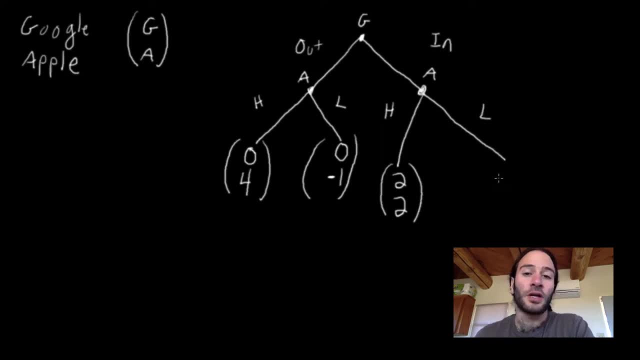 However, if Apple chooses a low price, it's essentially entering a price war with Google, and they'll both get negative one. Well, we'll say they'll get negative two. Price wars are bad for companies. Okay, so this fully represents the game. These here are called decision nodes. 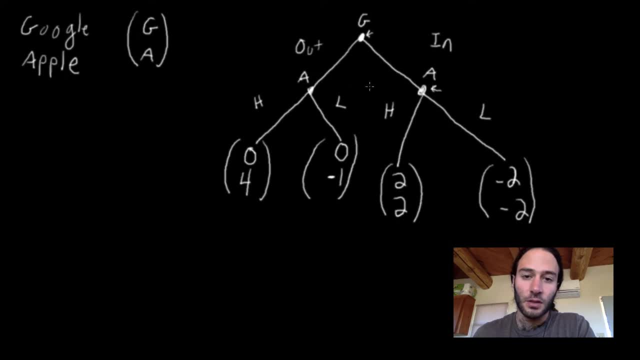 This is Google's decision node. This and this are Apple's decision nodes. Now, before we talk about solving this game, let's write out the strategies. So what is a strategy for Google? Remember, a strategy specifies what a player would do at each of its decision. 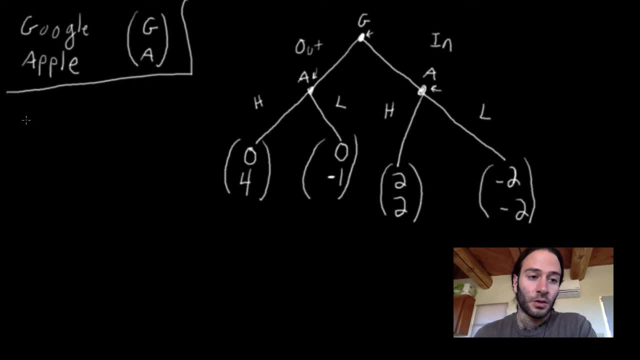 nodes. Well, Google only has one decision node, so strategy for Google- we'll call it SG- is either in or out. How about the strategy for Apple? I'm going to write this down here because we're going to need some room. So remember, Apple has to specify what it would do at each of its 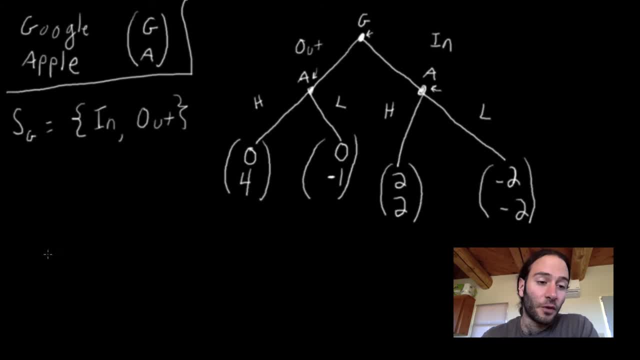 decision nodes. So Apple's strategy is of the form: if Google plays out, then do something. If Google plays in, then do something. Okay, So what are the different strategies? Well, if Google plays out, Apple can play a high price, and if Google plays in, Apple can. 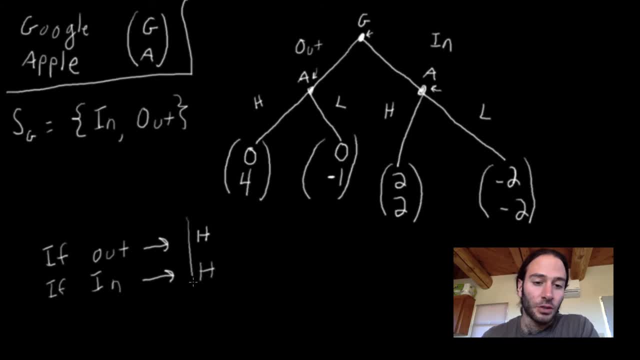 play a high price. So this HH is one strategy. If Google plays out, charge a high price. If Google plays in, charge a high price, Another strategy can be this HL. So I'm writing it like this so I don't have to keep writing: if out, if in. 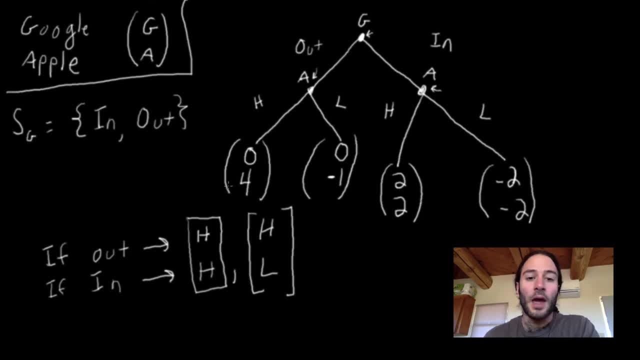 But the interpretation now is: if Google plays out, Apple plays a high price. If Google plays in, Apple plays a low price. Okay, And then of course we have the strategy LH: If Google plays out, Apple charges a low price. If Google plays in, Apple charges a high price. 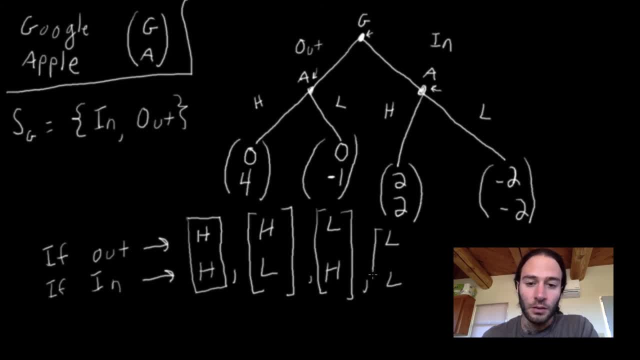 And, of course, the strategy LL. If Google plays out, Apple charges a low price, and if Google plays in, Apple also charges a low price. So we see, in this case Google has two strategies, but Apple has strategy one, two, three and four. So this is the full definition of the game, The tree here.